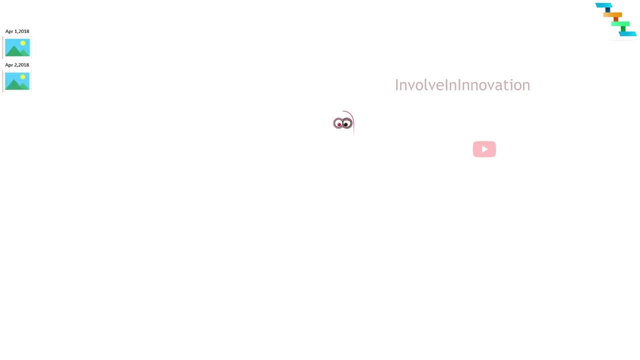 with version control. Version control is a system that records changes to a file or a setup file over a time so that you can recall specific versions later. Version control is also called as revision control or source control. For example, you are editing an image today and opening it. 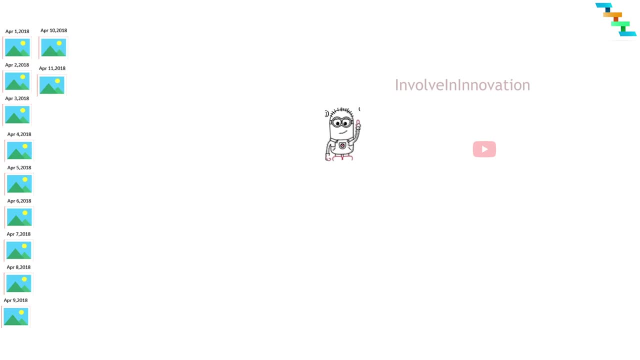 tomorrow, and then you need to edit the image in the next day or so, So you need to know what's going. making some more changes, then you feel like you messed up something today and we want to go back to the previous version which you have saved yesterday. 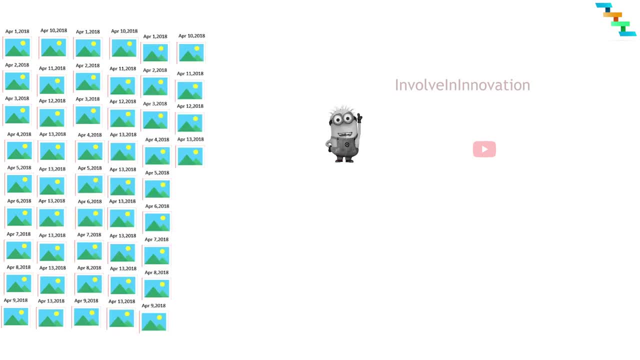 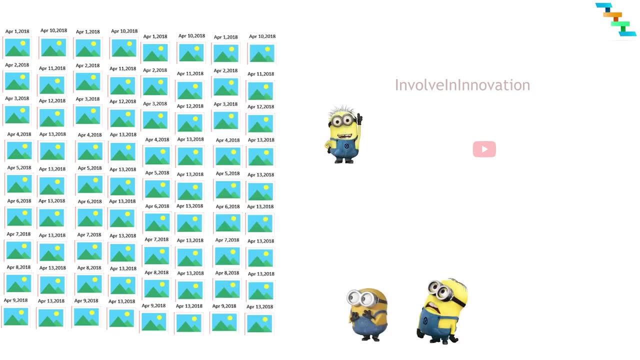 one way to handle this without version control is save each version daily, make a copy of yesterday's version and work on it. this will work well if you have minimal change. and what happens if you are working on a very big project which spans over a year and daily you want to create multiple versions and one biggest? 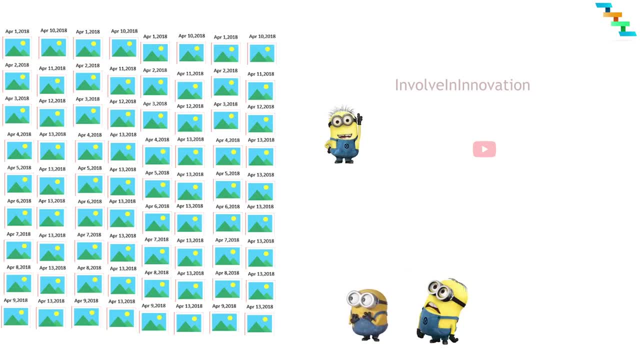 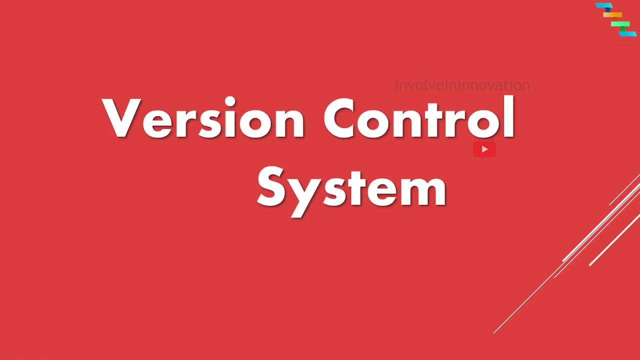 problem is it will become clumsy and data size increases. what if multiple people want to contribute to the same project? this is where we need version control and, provided we are working remote now, the version control tool is mandatory if you are a graphic or web designer or a software engineer and want 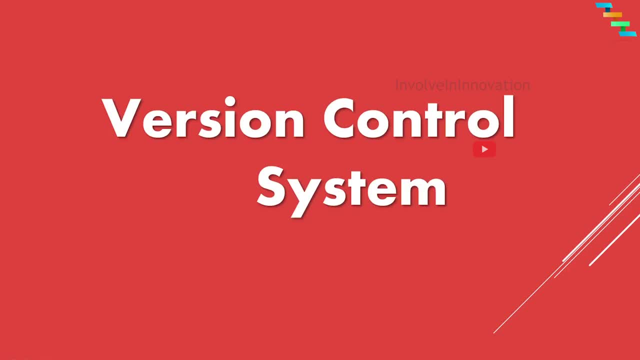 to keep every version of image or layout or code base which you would most certainly want to. a version control is very wise thing to use. it allows you to run a lot of code in a very short period of time. so if you are working on a reverse version of an image or layout or code base which you want to use, it allows you to. 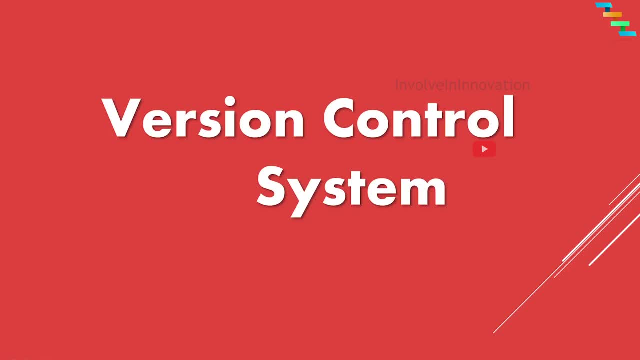 revert selected files back to a previous state. revert the entire project back to the previous state. compare changes over time. compare between different branches and see who last modified something and that might be causing a problem. who introduced the issue when and more. using a version control also means if you screw things up or lose files, you can easily recover. 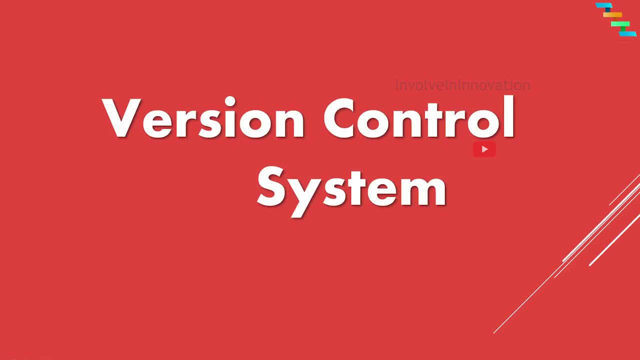 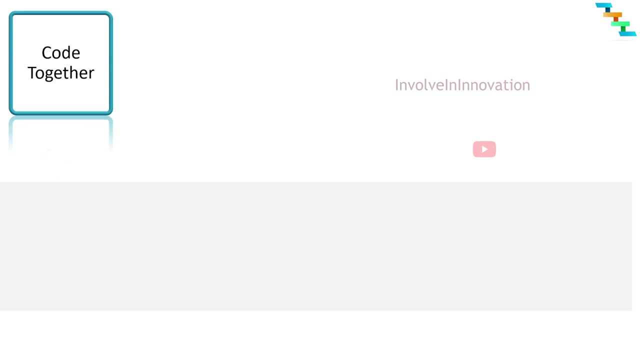 in addition, you will get all this with a very little overhead. there are lots of benefit if you use version control system. now we'll discuss about some of the key important benefits. first thing is co2 weather. now, in current world, co2 weather is very essential because you are from any part in the world. 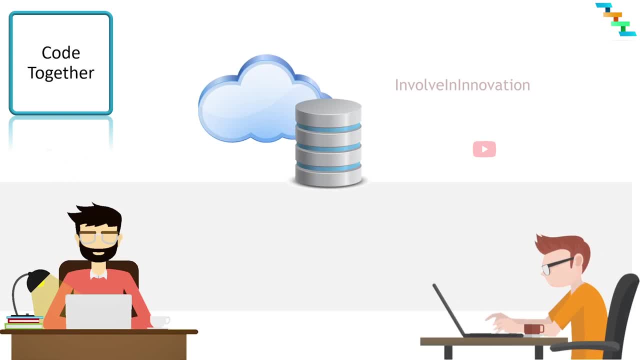 version control synchronizes versions and make sure that your changes don't conflict with other changes from your team members. your team relies on version control to help resolve and prevent conflicts, even when people change their at the same time, so developers can work remotely and still make sure that the 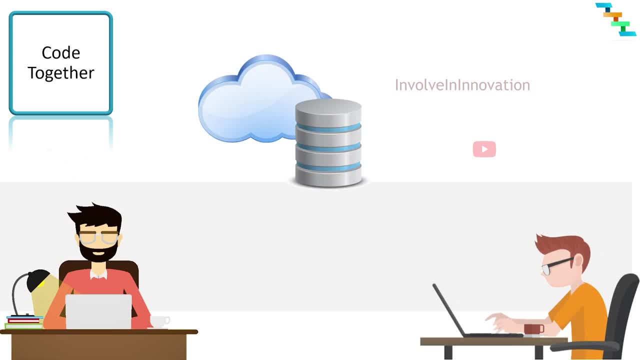 changes are not conflicting with each other and they can work on same feature parallelly. if there is a conflict, they can resolve at the earliest stage possible. for example, there are two developers who are working on the same project. one developer commit the initial version to the remote repository and 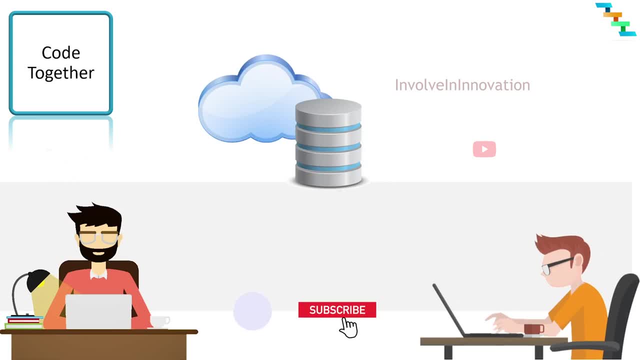 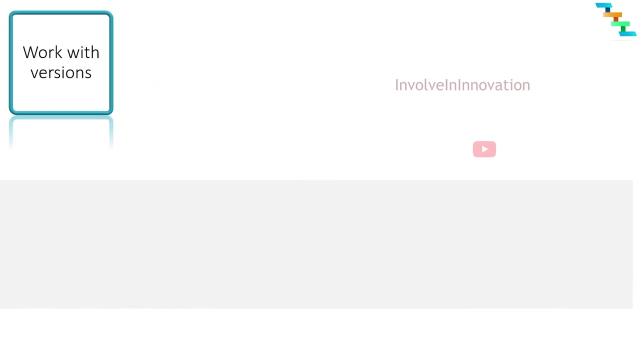 another developer, who can be working from a different geographical area, can take this file and modify this file and push it back to the same remote repository. by this way, they can code together on the same code base using this version control tool. next is versioning- think the software which you 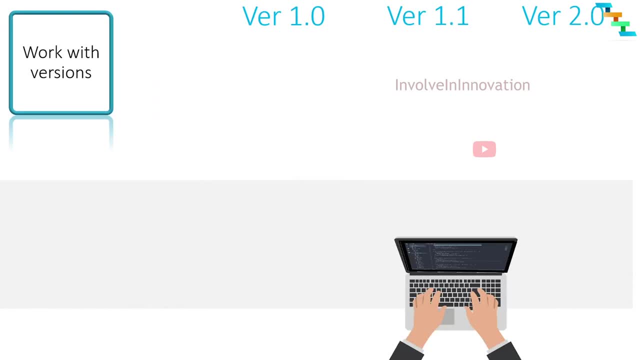 are creating as different versions. in this case, you can easily create multiple branches and that multiple branches can support different versions. so version control allows you to save changes to each version individually and without affecting other versions of the version control tool. so if you want to save changes to each version, you can save changes to each version individually and without affecting other versions, and you will also work on multiple. 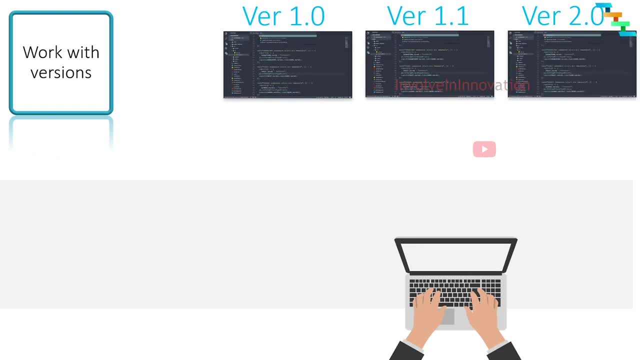 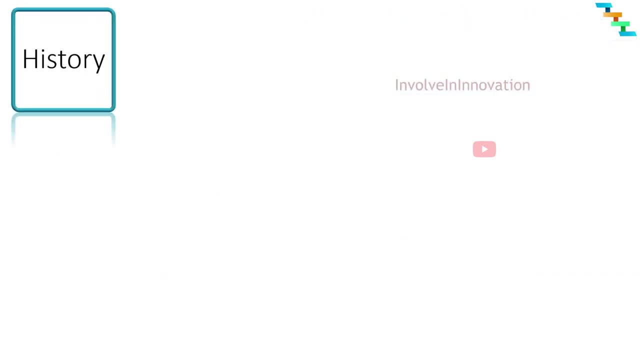 versions parallelly. you no need to wait for one version to go to production to work on the different version. next important thing is keeping a history, version control tags, the history of changes as your team saves new version of code. this history can be used to find who, when and why changes are made and 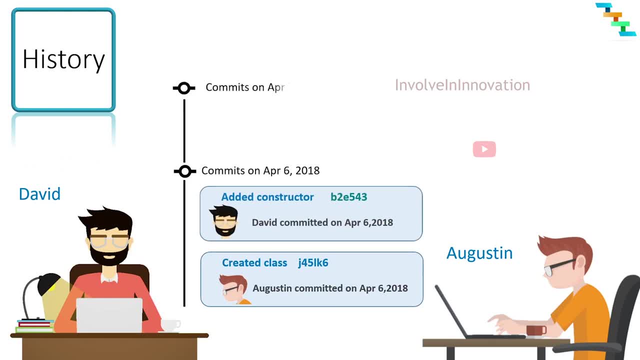 even what changes are made. history gives you the confidence to experiment, since you can roll back to any previous good version at any time. history lets your base work from any version of code, such as to fix a bug in the previous release, for example. here there are two. 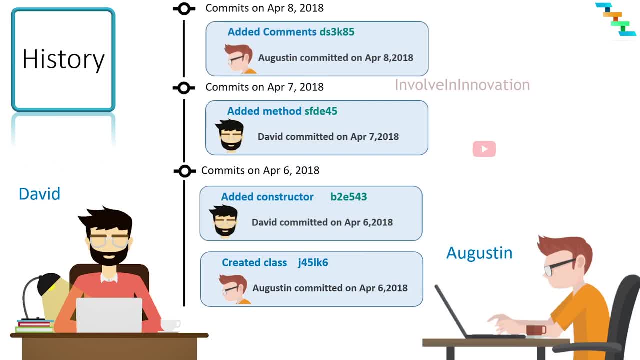 developers who are working remotely. each commit made by a developer has the information such as when the commit is made, who did the commit and descriptive message: developer added to the commit: change history and unique commit hash. we also have some of the very important benefits in today's version of code. let's 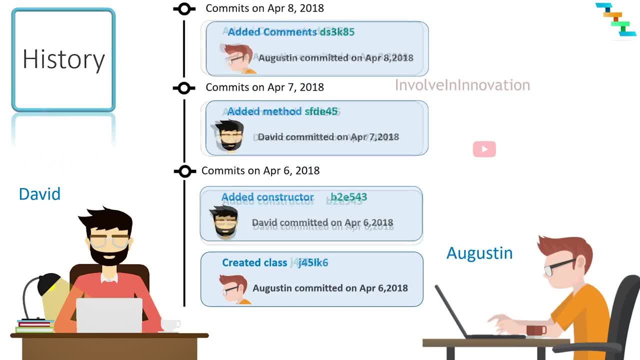 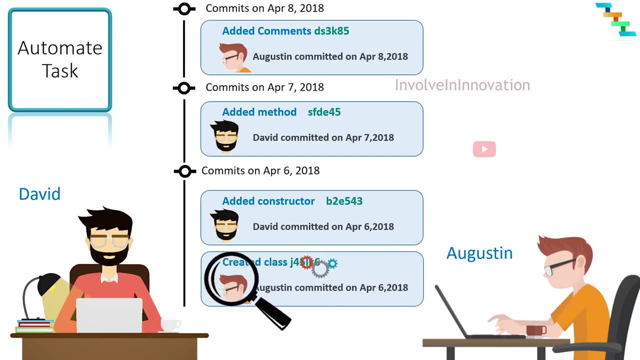 world. that is CICD Version control automation features. it saves your team time and generate consistent results. Automate unit testing, static code analysis, security vulnerabilities at the earliest stage possible and deploy, when the versions are saved, to version control, and you can even set up your own. 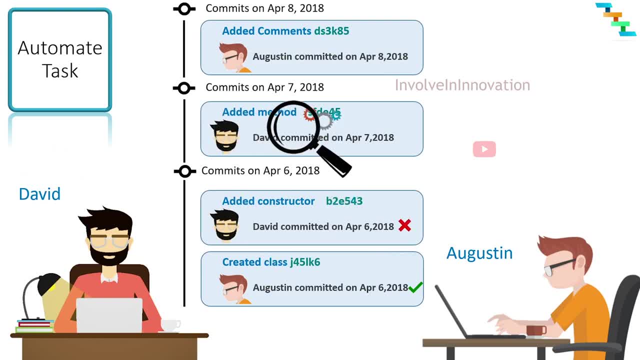 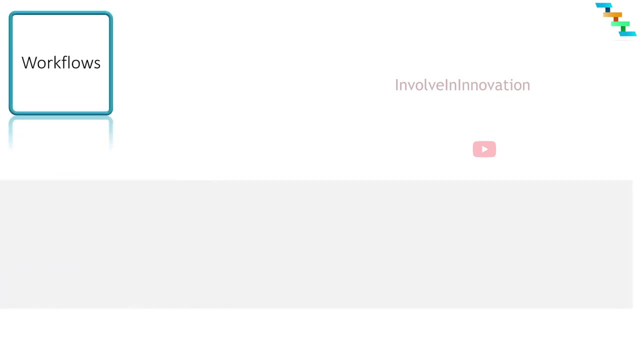 continuous integration and continuous deployment to a code base, so that whenever user commits to the particular branch, it will be deployed to any environment possible and you can also automate different tasks whenever a user commits to the repo Workflow. Version control workflows prevent the chaos of everyone using their own development process with different and incompatible 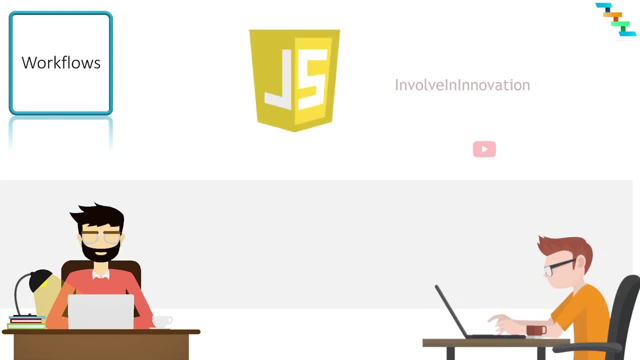 tools. Version control system provides process enforcement and permissions, so everyone stays on the same page. For example, let's consider two developers working on a JavaScript project for which they are not using version control. let's take one using CICD, One using Gulpjs to automate time-consuming task and another one using 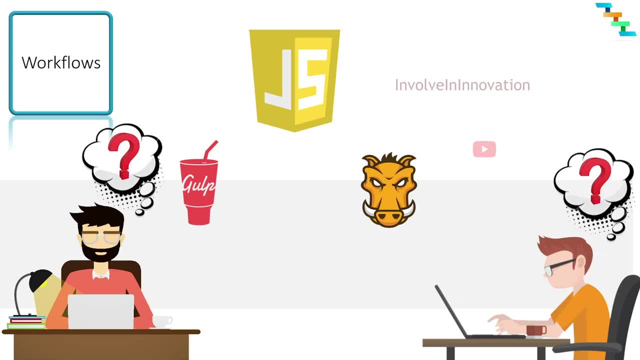 Grunt to automate time-consuming task. Now, when they want to merge their code, they need to use not two but one, so it requires substantial changes to unify the project to same tool. This can be avoided easily if everyone is using version control from the day one and version control avoids this kind of conflict. 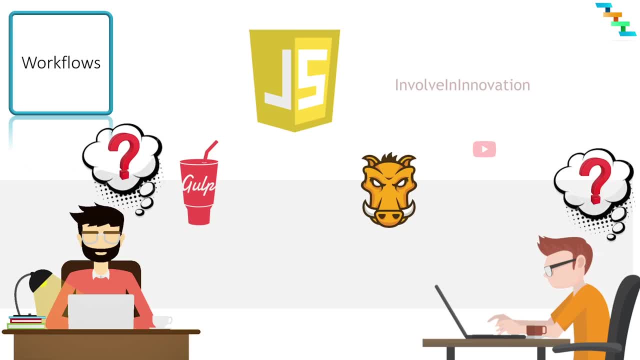 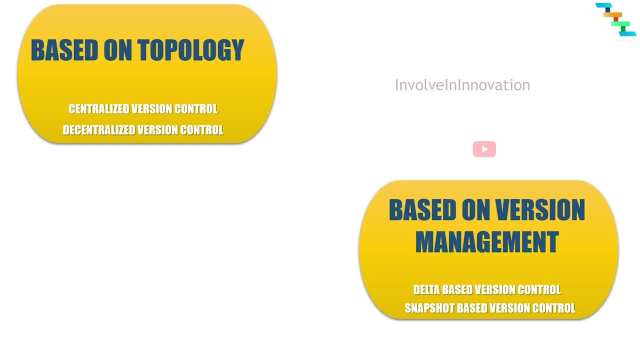 Next we will see about two major divisions of version control control. there are two major divisions: one based on the topology of project and another based on how we represent the versions. based on topology, it is divided into centralized version control and decentralized version control. centralized version control systems are based on the idea. 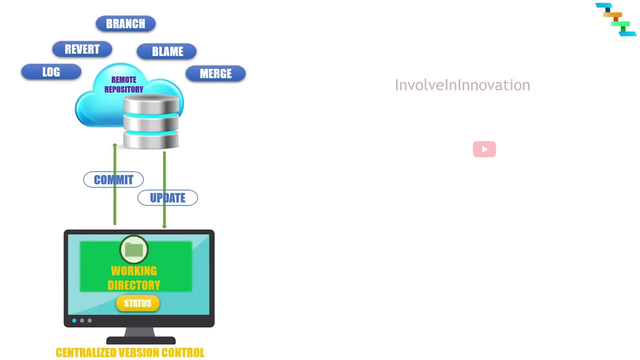 that there is a single central copy of your project somewhere probably on the server, and programmers will commit their changes to the central copy. committing a change simply means recording the change in the central system. other programmers can see this change here. check out means taking the latest version of code from the central server and history will be. 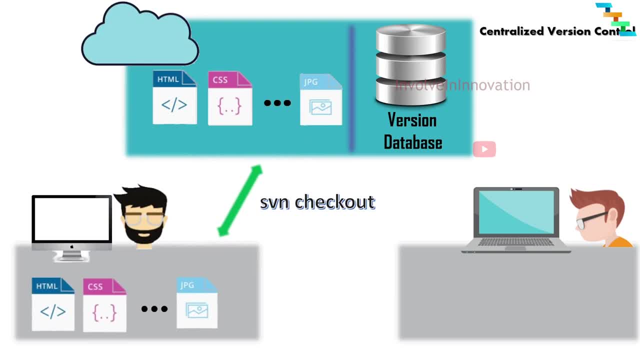 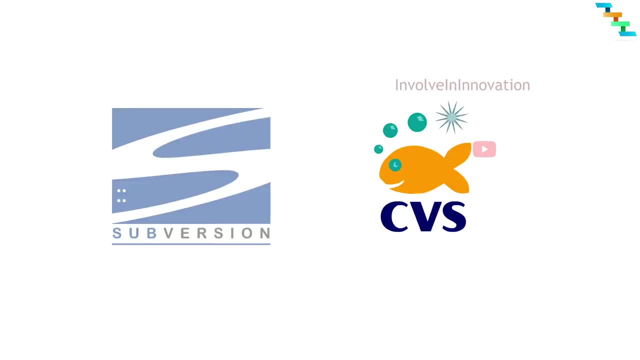 always preserved in the server. only if server data gets corrupt, the user cannot get the history of files. example of centralized version control systems are svn and cvs. people are not using centralized version control system. much people have moved towards decentralized. there are several centralized version control systems that are based on centralized version control system. 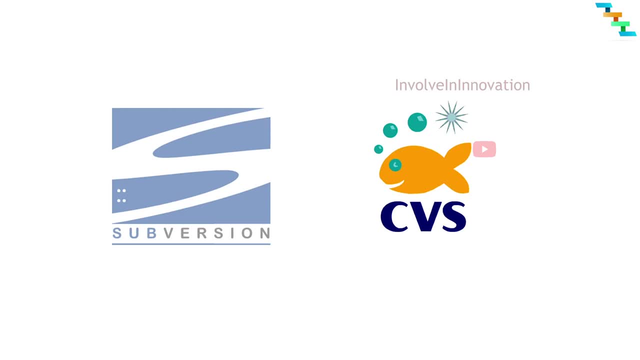 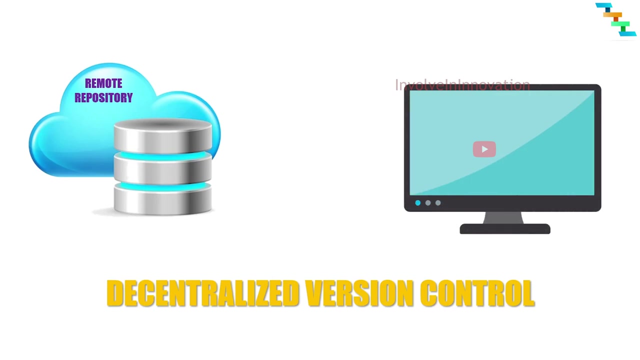 some legacy applications still using svn. so understanding svn also vital if we are supporting a legacy project. next we will see about decentralized version control. decentralized version control system do not necessarily lay on a central server to store all the versions of a project file. instead, every developer machine clones a copy of a repository. 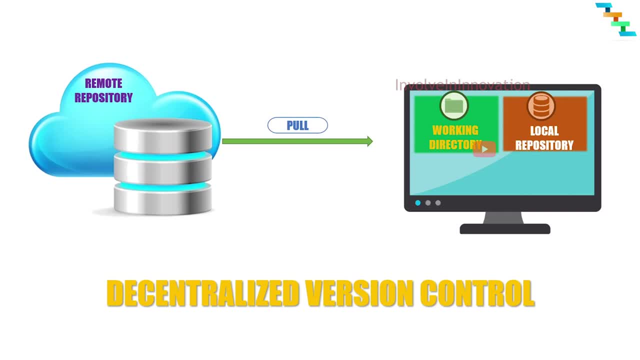 and has the full history of the project on their own hard drive. this copy, or clone, has all the metadata of the original. the act of getting new changes from a repository is usually called pull, and the act of moving your code changes to this repository is push in both cases. 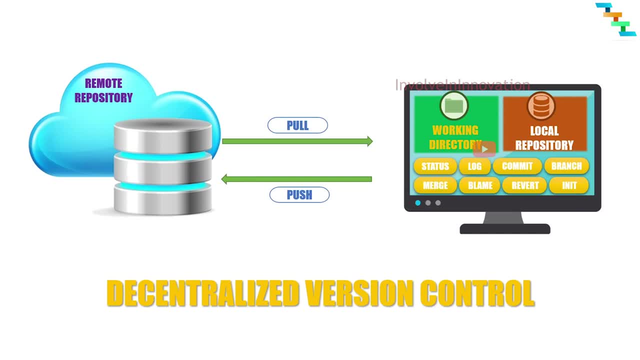 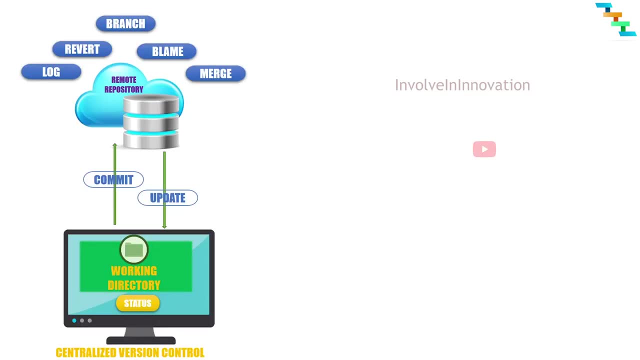 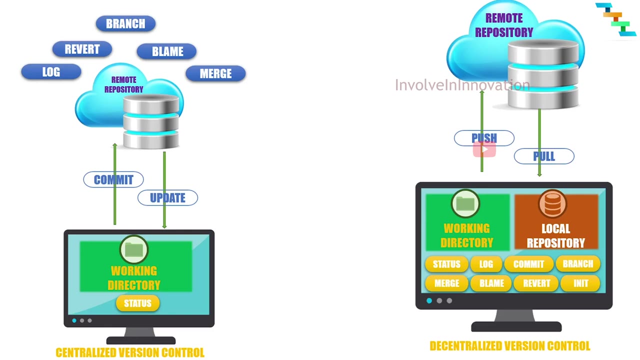 you move change sets, that is, changes to file groups as a coherent holes, not single file difference. advantages of using decentralized version control: performing actions other than push and pull change sense is extremely fast because the tool only needs to access the r driver, not the remote server. so for push and pull you need active internet connection. 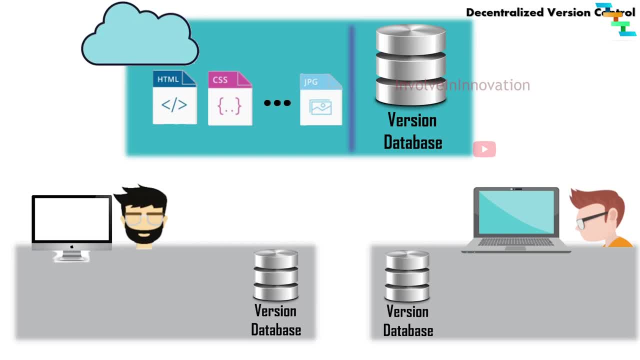 if the server is down or server data get deleted, the developer will have the history of files in the local. one developer can clone a version from other developer since you have history of files in their hardware. examples of decentralized version control systems are git and mercurial. now you will see, based on how we represent the version it is divided into, 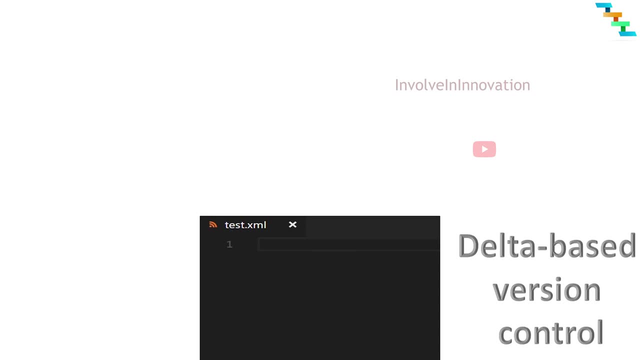 delta based version control system and snapshot based version control system. delta based version control system store information as list of file based changes. this system thinks information restore as a set of files and changes made to each file over time. this is commonly described as delta based version control, so we will see this with the example. 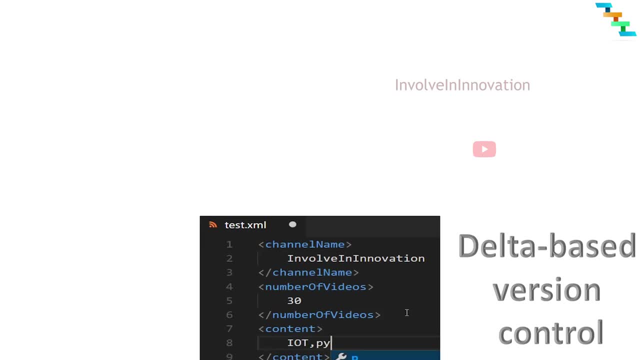 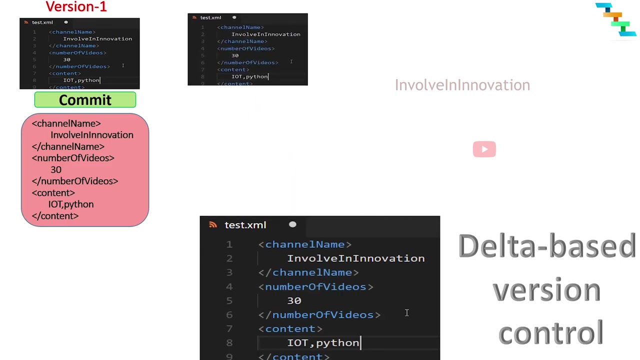 here i am creating a file named test dot xml. i am committing this test dot xml for the first time, so this is the initial version. first, it stores the complete tested dot xm file. i am committing again, without doing any modification to the test dot xml. this will be stored as the version two. in the version 2, no code changes are stored. 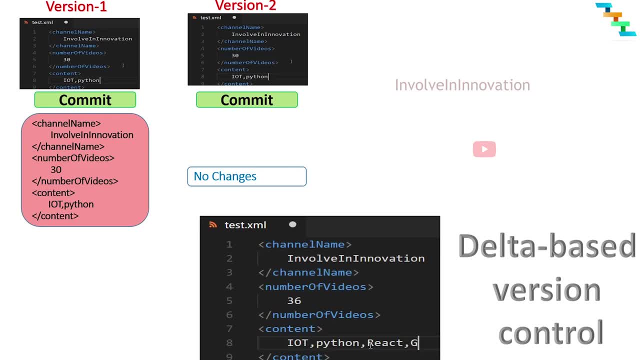 now i made some changes to the tested root exome and committing it again. now it is stored as version two. only the modified information is stored here. 36 got replaced with 40, the delta as 36 as deleted and 40 as added, and i added react and git to the content. so it is stored. 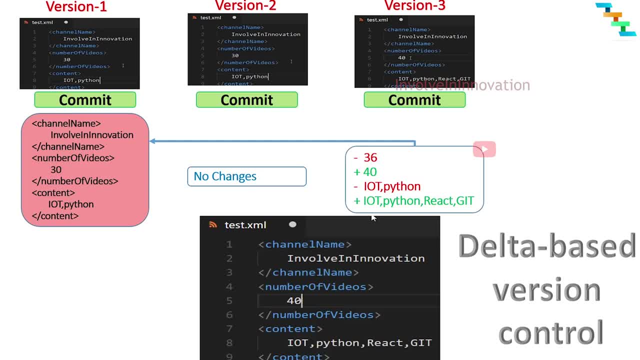 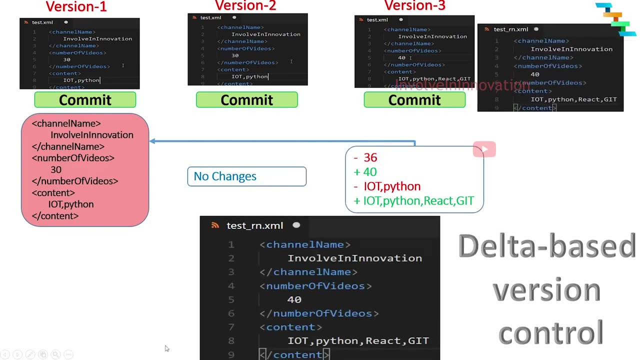 the delta as iot python, react git as newly added and iot python got deleted in the delta based version control, not storing the full file, only the changes are stored as the delta. now if i rename the file testxml to test underscore rn dot xml, it will be stored as file rename and this will 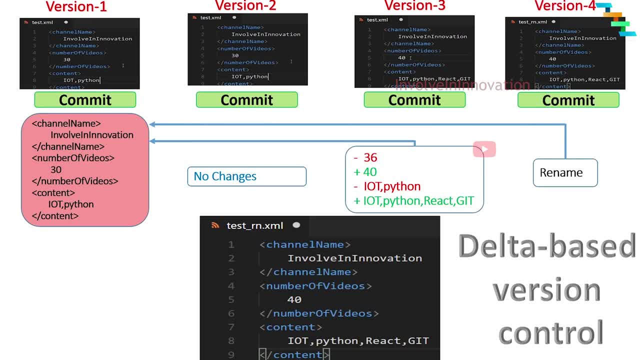 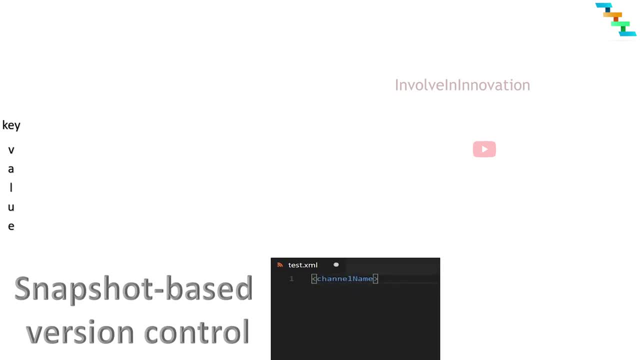 point to the original testxml. what is snapshot based version control? this system thinks of its data more like a series of snapshots of a miniature file system with snapshot based version control. every time you commit or save the state of your project, it basically takes the picture of what all your files look like at that moment. 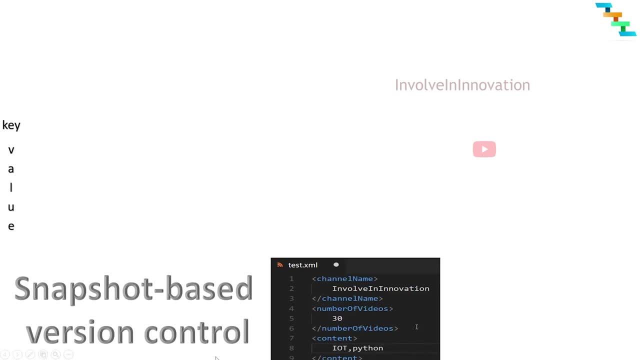 and stores a reference to that snapshot to be efficient. if the files have not changed, it does not store the file again, just a link to the previous identical file it has already stored. git thinks about its data more like a stream of snapshots. we will see this with the example here. 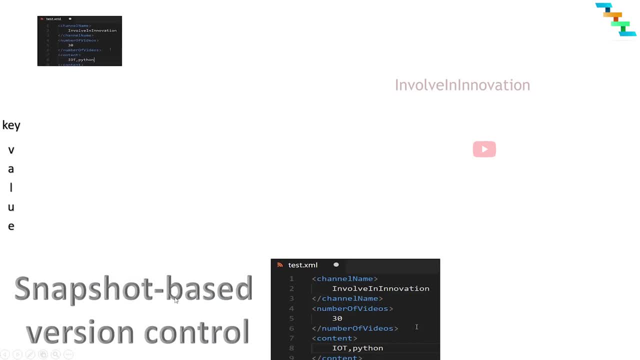 we have the same testxml and i am committing its initial version here. it got saved as complete file with a unique hash code. for the sake of simplicity, let's take the commit hash as x8n, so this is the hash code here. x8n hash key holds the complete file. 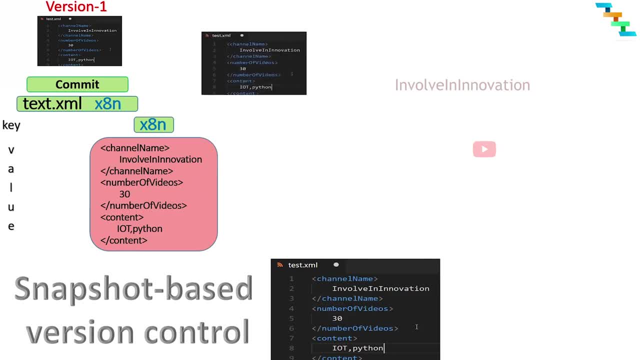 information. i am committing the testxml again without doing any modification. so now in the version 2 we have same commit hash for the file, which refers to the initial version of the file. i am committing another version by adding some modification to the textxml. now this will store the complete file with a new hash code. this is the. 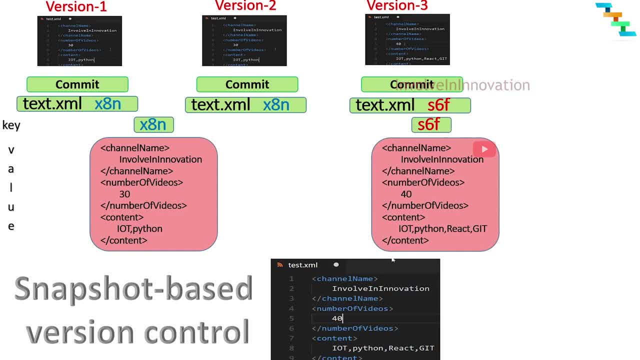 main difference between snapshot based version control versus delta based version control. as we seen in the delta based version control this got saved as a delta file difference, whereas here in the snapshot based version control, it is saved as a complete file with a different hash code representing this commit. if you rename this file from testxml to test underscore rn xml. 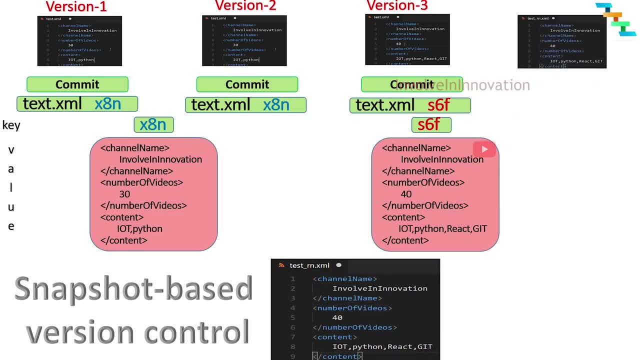 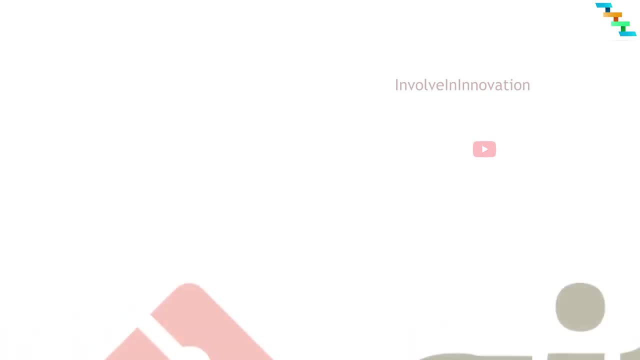 the file got renamed, but it still points to the previous commit hash. if you are familiar with git, we will find some discrepancies here with the file name. we will cover more about this when we discuss git mv command in the coming videos. next we will see why we need git. git is the most commonly used. 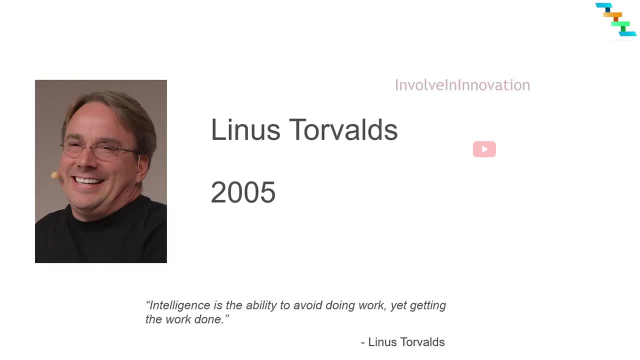 version control system. today, git is mature, actively maintained open source project originally developed in 2005 by linux star wars, the famous creator of the linux operating system kernel. a staggering number of software projects on git version control system. You may be very familiar with github, gitlab, bitbucket. 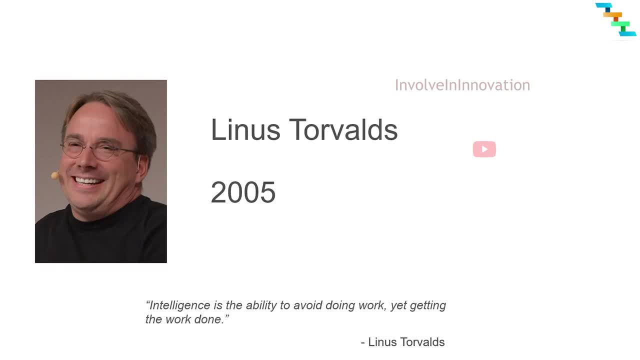 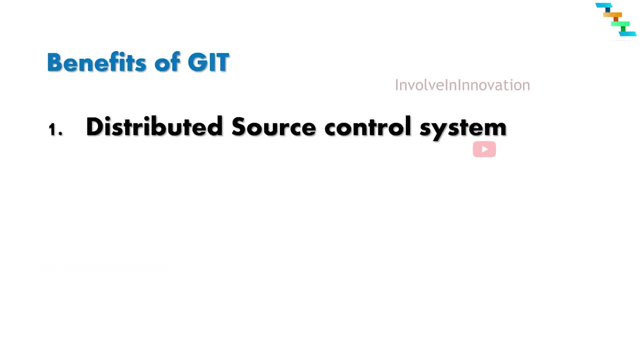 all those are laid on git technology, including commercial projects as well as open source. These are important benefits of using git. Git is a distributed source control system and snapshot based version control system. Git does not necessarily lay on central server to store all the versions of a project's files. Instead, every developer clones a copy. 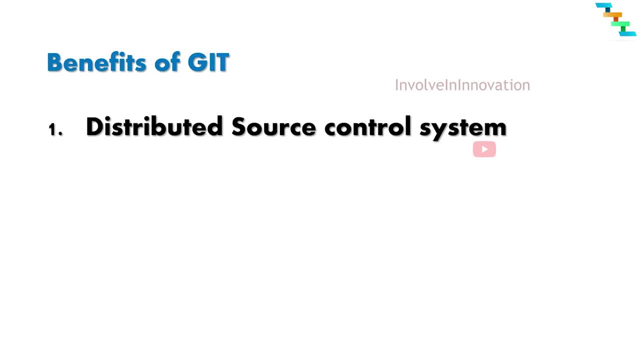 of a repository and has a full history of the project on their own hard drive. Git scales massively. Because of the distributed nature of git, it can scale massively. Git is initially developed for Linux project requirements. Today, Linux kernel has over 15 million lines of code and more than 1200 developers across the globe, And git is free. 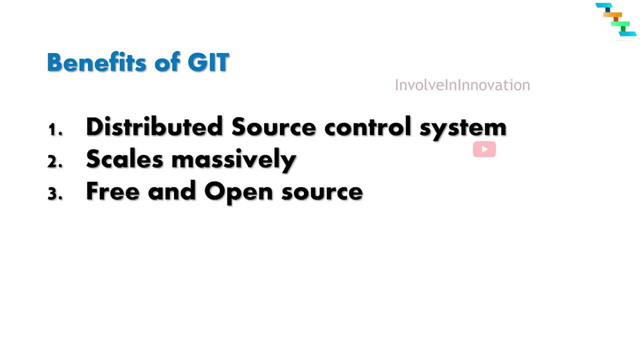 and open source. There are many commercial projects which are based on git and you can also find free and open source system which are based on git. One great example is github. Because of its distributed nature, most operations in the git are local, So you might not need active. 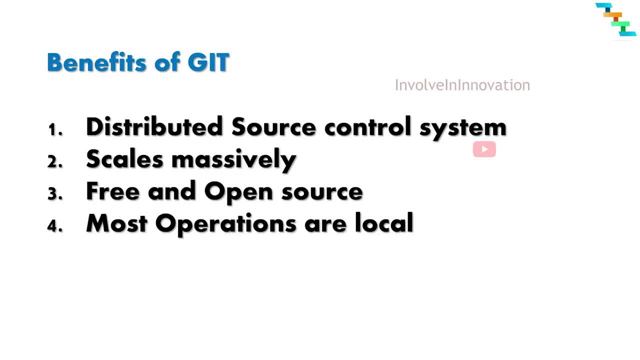 internet connection most often. Git has a very active community and it is evolving day by day. It has already become mature, but it is evolving day by day, so that most of the answers which you are looking for is already answered by you. Now we will see about some of the key terminologies and basics about git. 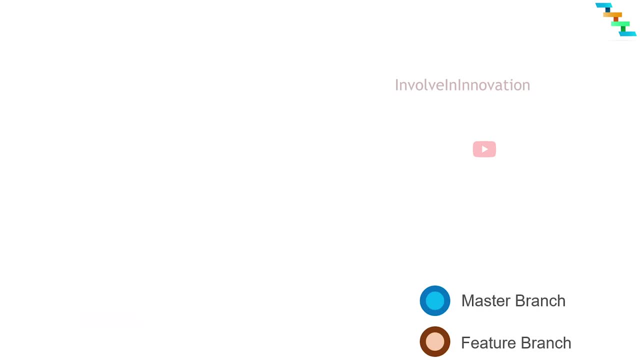 Every time you save your work, git creates a commit. A commit is a snapshot of all your files at a point in time. If a file has not changed from one commit to the next, git uses a previously stored file. Commits create links to other commits, forming a graph of your 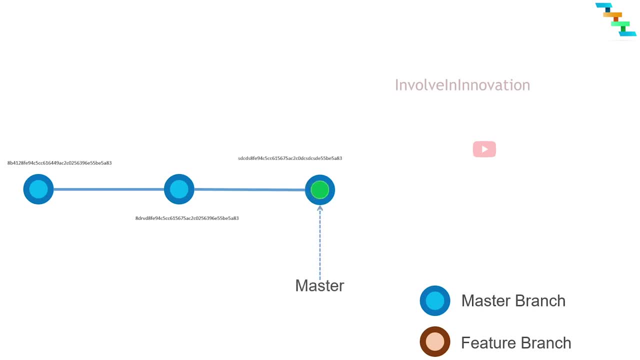 development history. You can revert your code to the previous commit, inspect how files changed from one commit to the next and review information such as where and when changes were made. Commits are identified in git by a unique cryptographic hash of the contents of the. 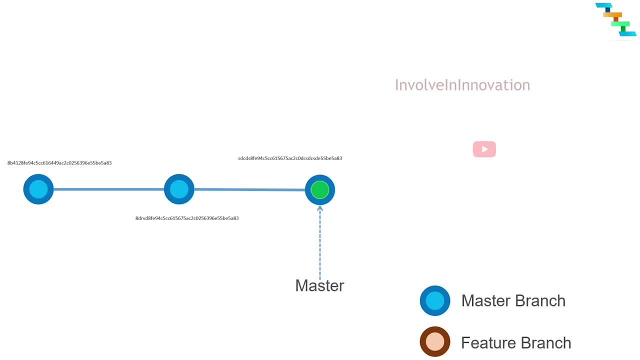 commit, Because everything is hashed. it is impossible to make changes or loose information or corrupt files without git detecting it. Now we will see about standard gems. The first is common: their own local code repository. as a result, you can have different changes based on the same commit. 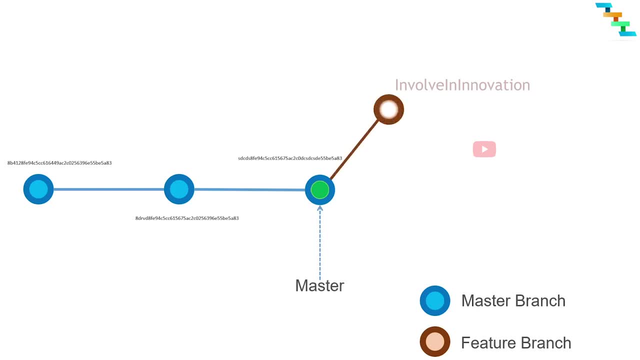 git provides tools for isolating changes and later merging them back together. a branch in git is simply a lightweight, movable pointer. a default branch name in git is master, but this is completely customizable. as you initially make commits, you are given a master branch that points to the last. 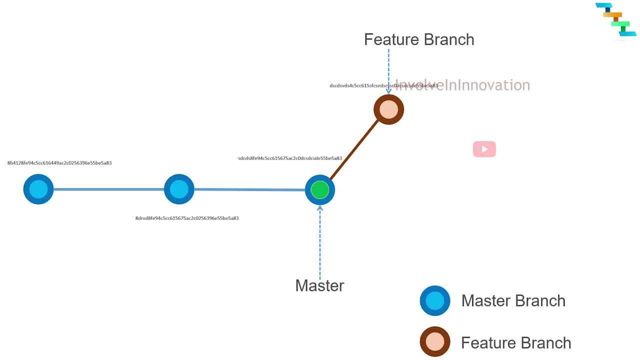 commit you made. every time you commit it moves forward automatically branches which are lightweight pointers, which is created for each and every feature or epic. once your feature or epic is completed and you have tested that feature, then you can move that branch to the team main branch. so here branches will be created for individual developers. so if the developer works on a 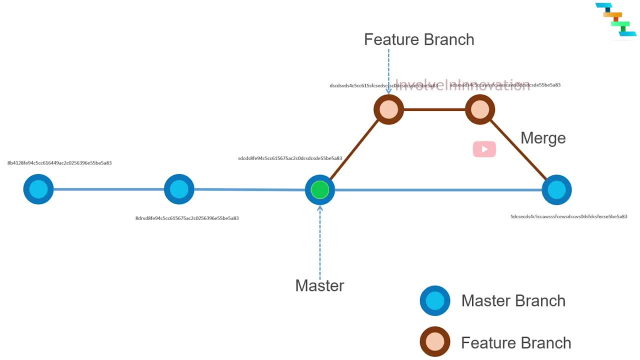 particular feature, he or she will create a branch tagging that particular feature. once that feature is done, he or she can merge it back to the master branch. files in git can be in one of the three stages: one is working directory, next is staging area and the third is the remote. 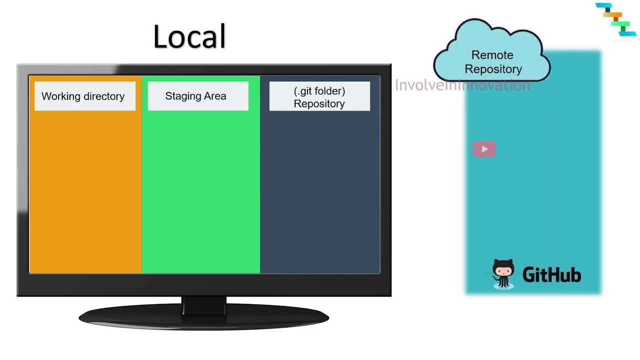 repository. when you first modify a file, the changes exist only in the working directory. they are not yet part of the commit or your development history. here i have created three files: a html, a css and a image file. in this working directory you must stage the files you want to include in your next commit. 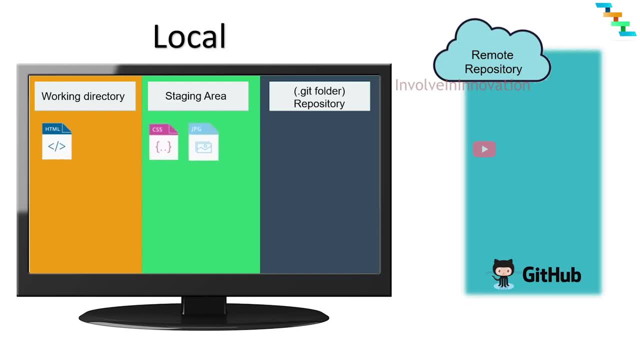 here. you can do that by using the command git add and pointing to the files you want to add to the staging area. and you can even omit files that you wish to commit separately by doing add with one file and then you can commit, and you can add another file and then you can commit. 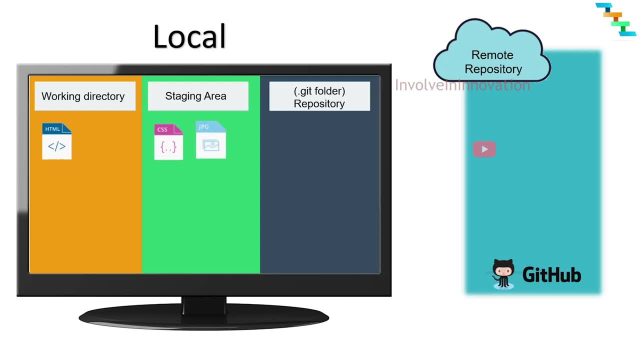 here. i want to stage only the css and image file so that it will be included in the next commit. the staging area contains all the changes that you will include in our next commit. once you are happy with the staged files, commit them with a message describing what changed. this commit message might be really important because this may be serve as a 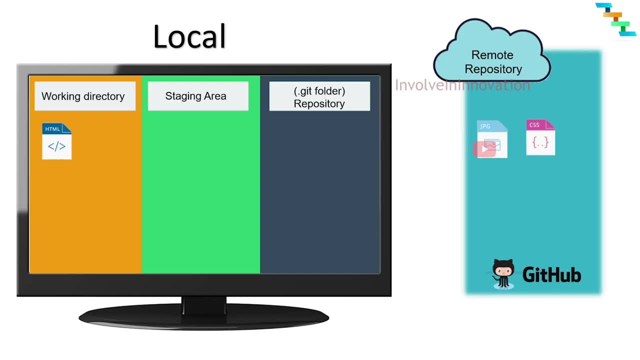 documentation for you and your teammates. this commit becomes a part of your development history here. when i hit the commit, the staged css and image files will be added to the next commit. now i am going to make a separate screen to actually do css and image photos here. 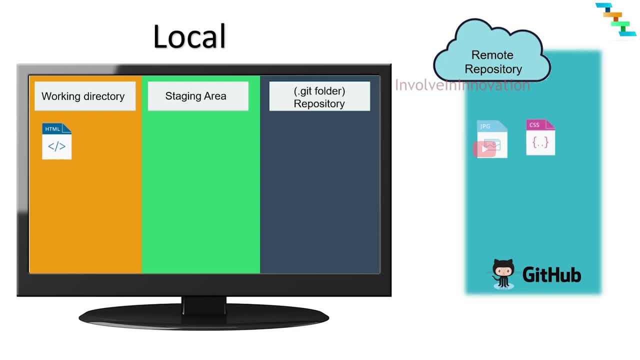 i am starting my next commit here and i am going to hate on the Strawaff. now, in the next video, now the next part, where we are going to create a new css and image file, and this is where we will need the neither when, yes, you are seeing theervil hl ochlihte. 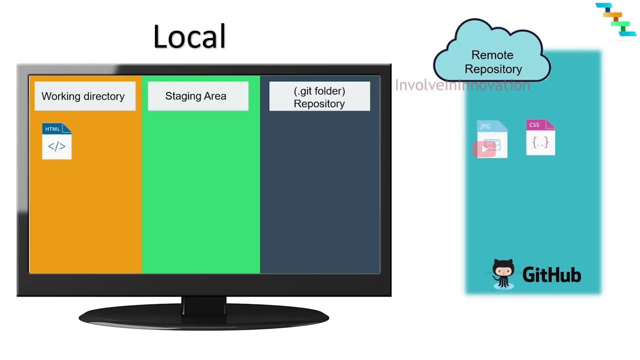 another common example here is when we have a localай 19.00 and, if need, we cannot infer any method, other two methods. however, in this case, what i have to do is add some code from my localai worksheets offline here. once you are finally okay with the changes, you can push the local commits to the 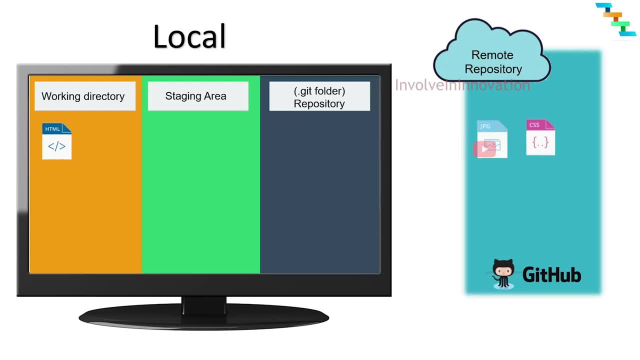 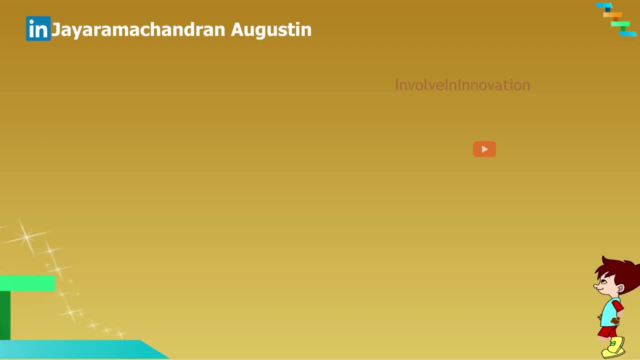 remote repository. this is when you need active internet connection because you are trying to contact the remote repository. i believe you have learned a lot in the first part of this git series. subscribe to this channel for more videos on git and hit like if you have enjoyed this content. 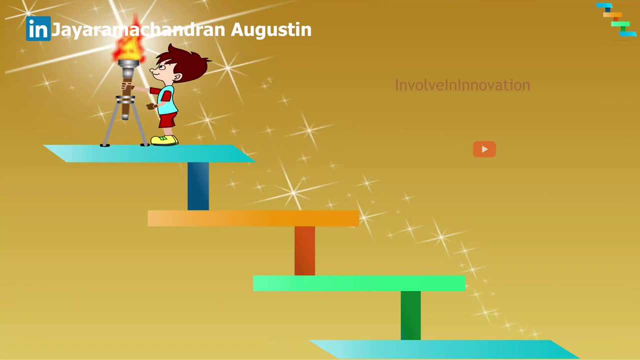 and share it with your friends. thanks for subscribing and watching this video.